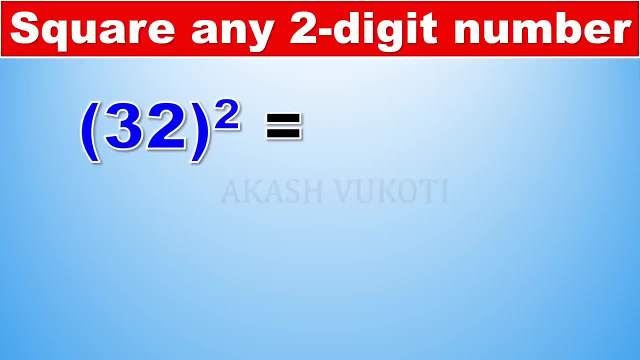 Now let's begin by separating the answer into three parts. The first part is just the first digit of 32 squared. So the first digit of 32 is 3, 3 squared is 9, and so 9 is the first digit. 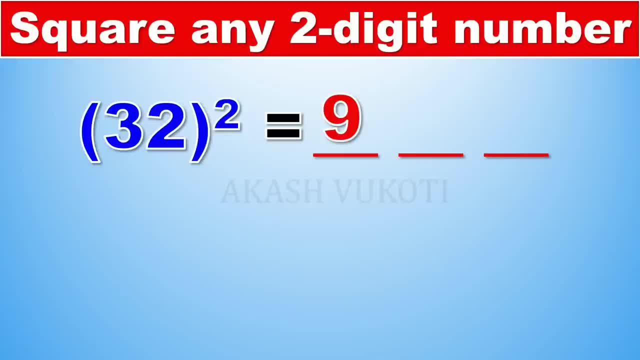 The last digit is just the square of the last digit of 32,, which is 2, 2 squared is 4, so 4 is the last digit of our answer. So now this is where it gets interesting, because the middle part is 3 times 2 times 2,. 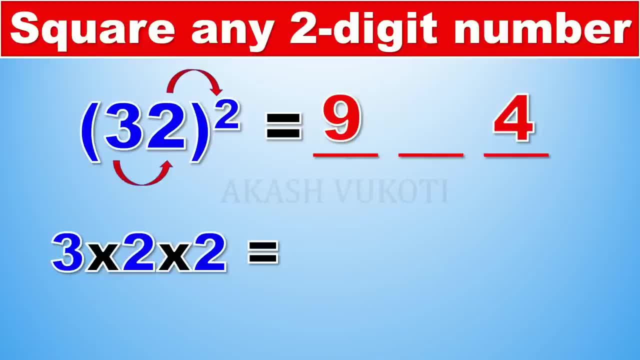 the product of the two digits of the original number multiplied by 2.. But the interesting thing is: 3 times 2, times 2 is 12, and 12 is a two digit number. So when we're calculating the solution, 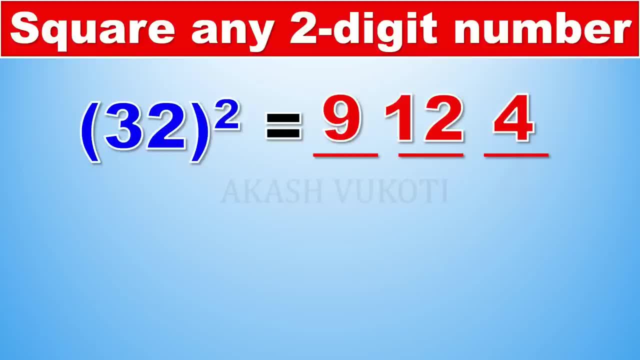 we're going to carry over. So let's take a look at what we have so far. The first part is 9,, the middle part is 12, and the last part is 4.. So, working from the last until the first, we have 4, and then we have 12,. 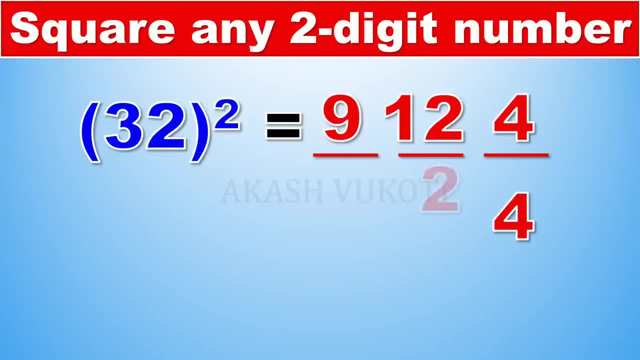 but we'll take the unit part of that, which is 2, and the 1 will be carried over to the next part, which is 9.. 9 plus 1 is 10, and so 10 is what we come out on the front. 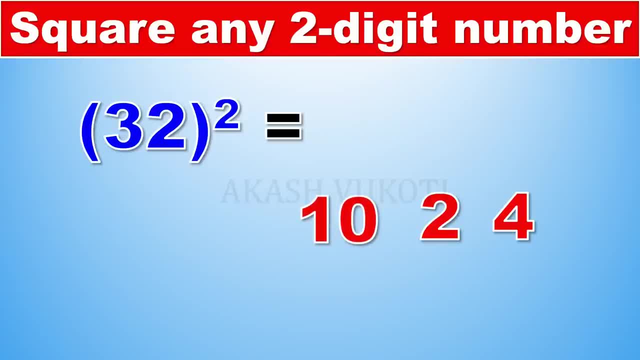 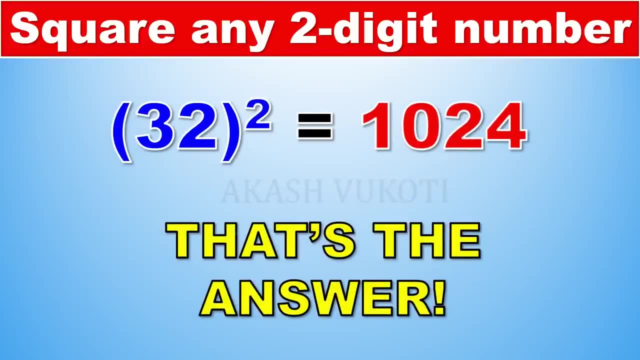 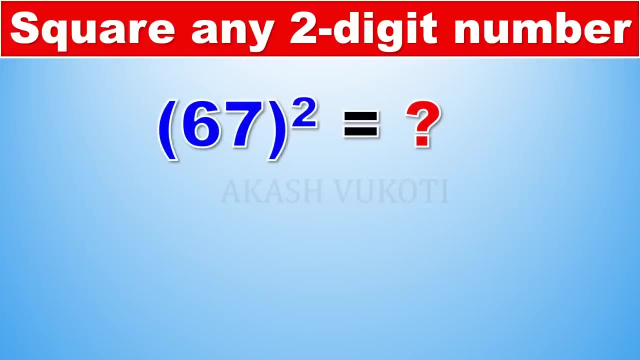 That means that 32 squared is equal to 1024.. Let's take a look at our third example. This one is quite a bit larger. This is 67 squared. Now we'll do the same thing that we did previously, So we start by dividing the answer into three portions. 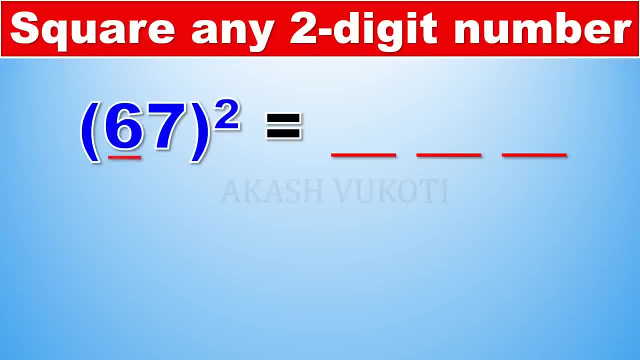 The first part is just the square of 6,, which is 36.. The last part is the square of 7, 49.. And so this is what we have so far. Now, the middle part is 6 times 7 times 2.. 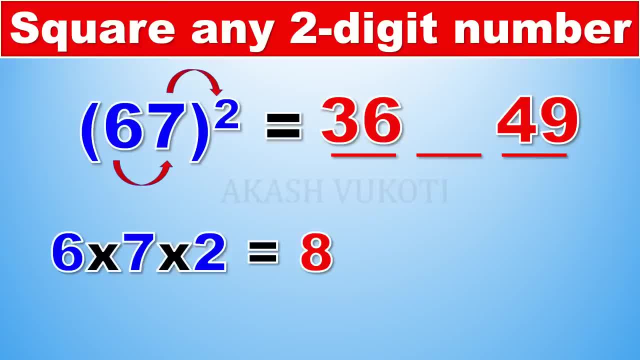 6 times 7 is 42, times 2 is 84.. And so now you have your three parts. So let's calculate the answer to this problem. And we begin, We start with 49.. And this already has two digits. 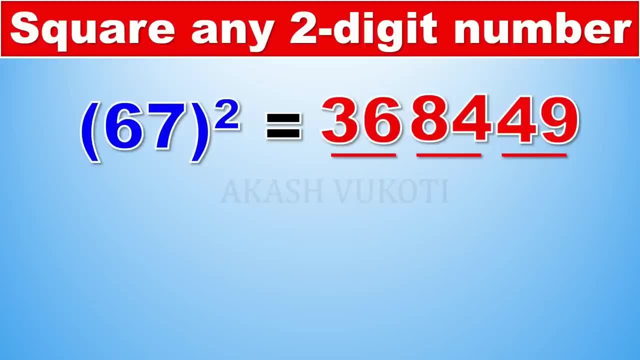 And we can only have one in this space. So what we do instead is just keep the 9 and carry over the 4.. Next we have 84. And 84 plus the 4 we carried from earlier is now 88.. 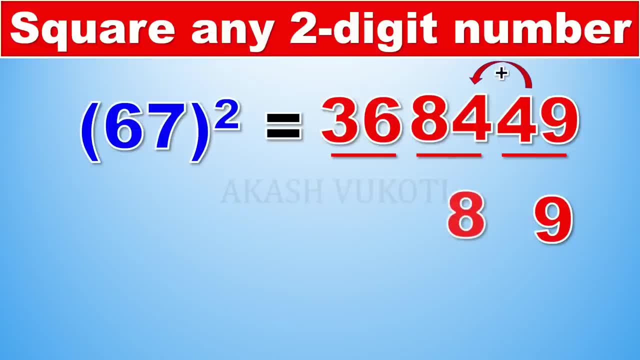 And again the same situation arises. We can only grab one, So we take the unit, which is now 8.. And that's the second to last digit of our answer. Then what we do is we take our 8 that we have left. 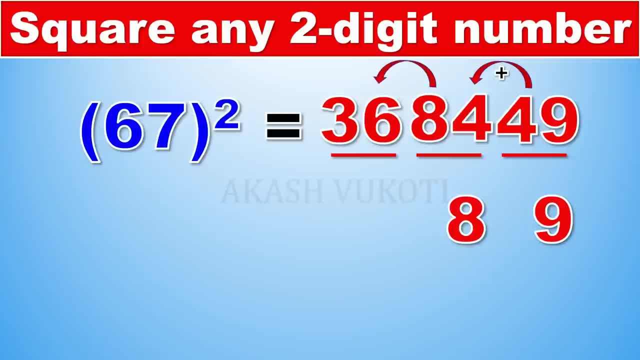 And we carry it over to the next part, which is 36.. And 36 plus 8 is 44. So then we just write 44 at the beginning, And therefore we have 67 squared equal to 4,489.. 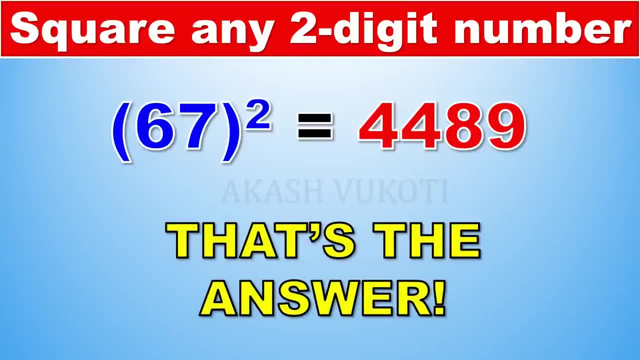 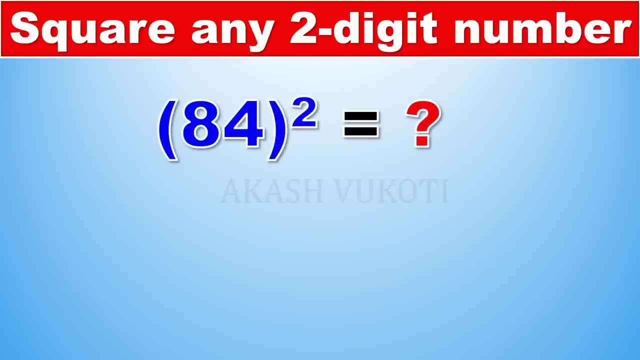 And that is the answer. Now let's take a look at one final example: 84 squared Now. by this time you'll be able to understand exactly what to do here. So we split the answer into three parts, Like we did with the other ones. 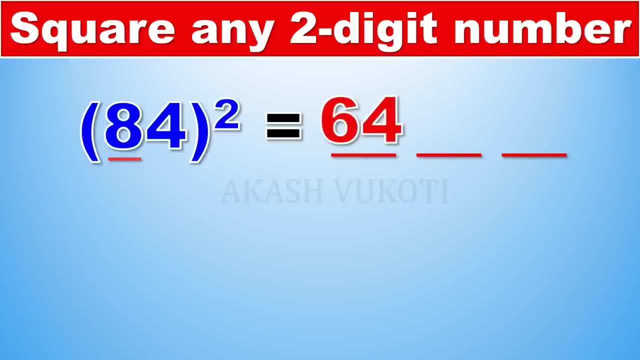 So the first part is 8 squared 64.. The last part is 4 squared 16.. And the middle part is 8 times 4 times 2.. Now we can just take a look: 8 times 4 is 32.. 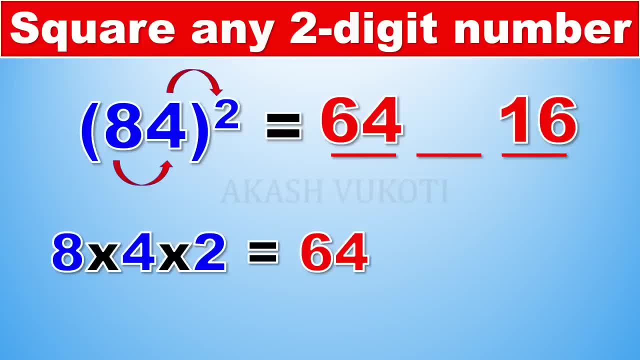 32 times 2 is 64. So 64 is our middle section And once again we can begin the process of carrying over all the digits. So we begin with 16.. Keep the 6. Carry over the 1 to 64..